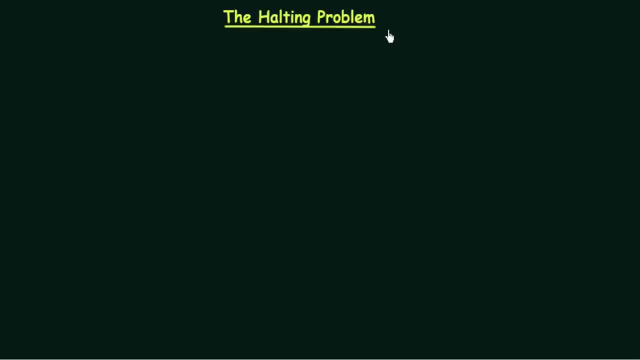 which is the halting problem. Alright, so first let's see what is this halting problem? So the halting problem says: Given a program, will it halt? So it is a question which asks that if we are given a particular program, 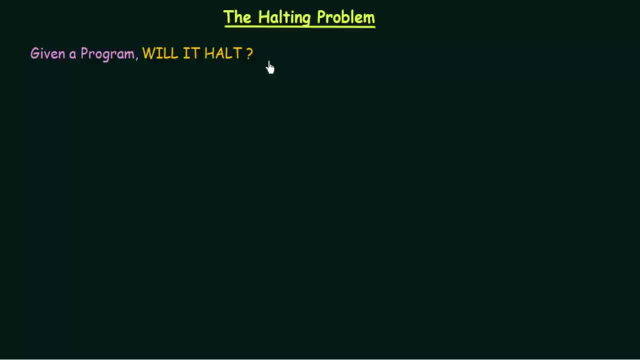 then can you make sure that this program will halt or not? And what do we mean by halting? Halting means that the program will either accept and halt or reject and halt, and it will never go into a loop. So that is what we mean by halting. 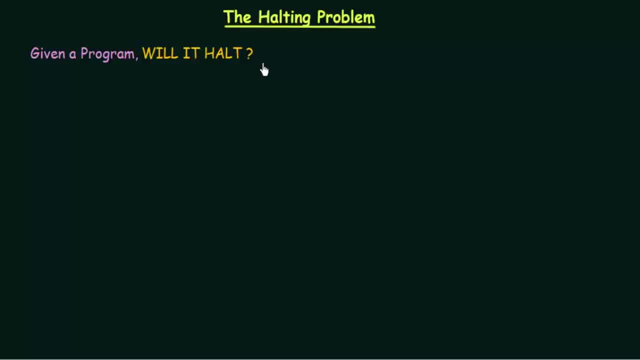 So can you have an algorithm that will tell you that a given program will either halt or not? Now, if you put it in terms of Turing machine, this is how you can ask the question: Given a Turing machine, will it halt when run on some particular given input string? 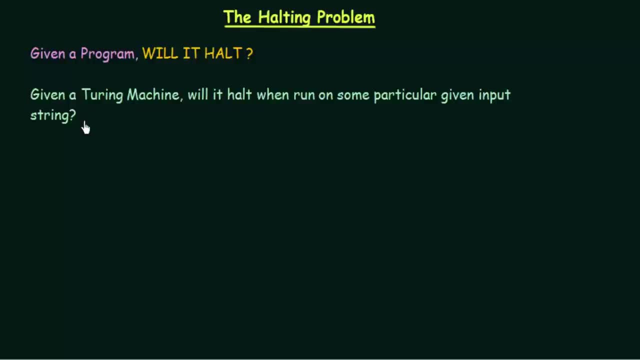 So if you have a Turing machine and if you give some particular input string to this Turing machine, will it halt or not? Now, if you think of any particular problem, we can say that by looking at the Turing machine or by looking at the program. 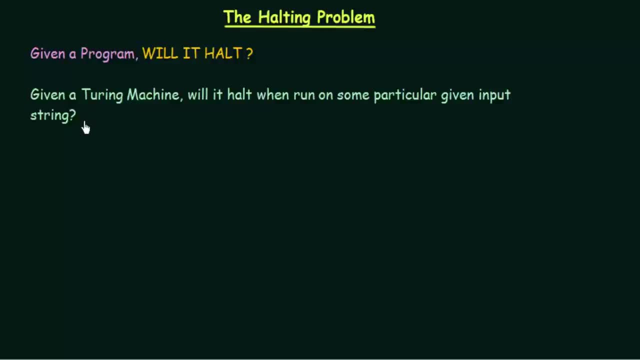 and the particular input that you give to the program or the Turing machine. you can say that, yes, this will halt, or this will not halt by the nature of it. But in a generalized way, will we be able to design a Turing machine? 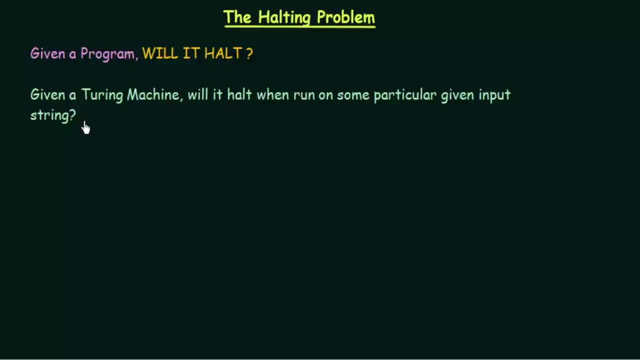 or an algorithm which will take any program and tell us whether that program will halt or not. So the answer to this is that no, we cannot design it. We cannot design a generalized algorithm into which, if we pass a program and then the algorithm tells us. 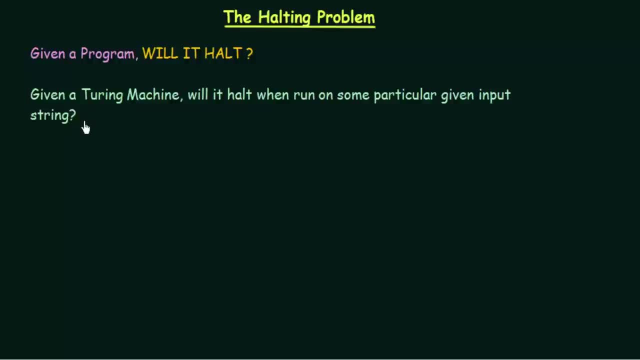 that this program will either halt or not. It is only possible to run the program with a particular input and then just see for ourselves whether it will halt or not. We cannot design something generalized. Now let us look at a similar question like this: 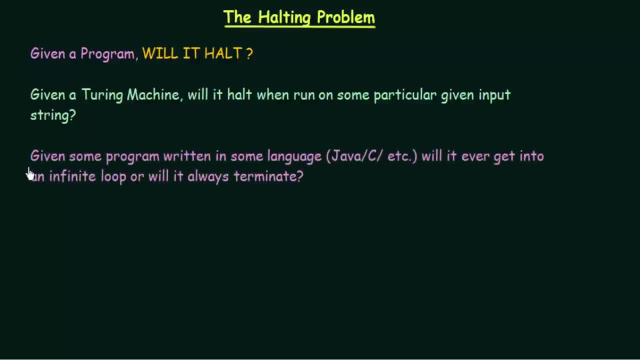 So here I can reframe this question in this way: Given some programs written in some language, let's say Java, C etc. Will it ever get into an infinite loop or will it always terminate? So if you have written some program, 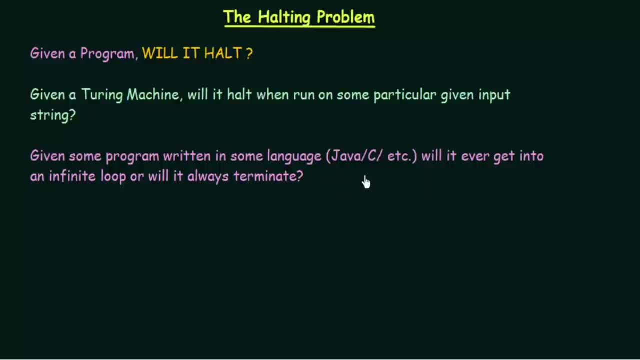 in any language of your choice, like Java or C, can you find out whether that program will go into an infinite loop or will it always terminate. So infinite loop means it will go into the looping state, and terminate means it will halt. So can you design a program like this? 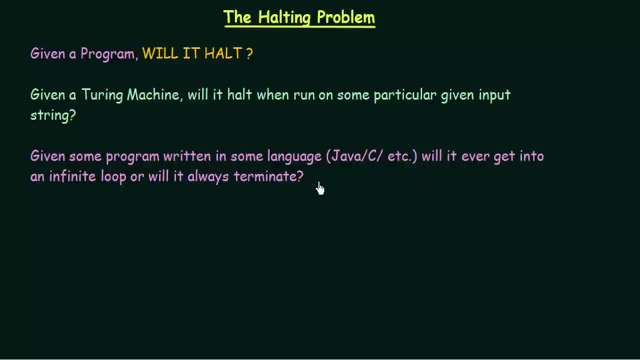 So can you develop an algorithm which will find out whether a given program will ever get into an infinite loop or it will always terminate? Now, if you remember, in the very first lecture of this lecture series, I took this example when I was giving you the introduction to: 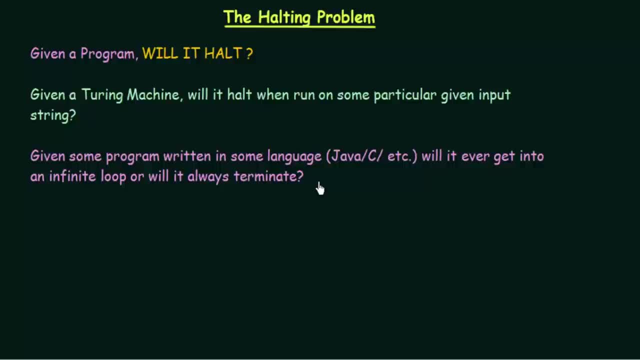 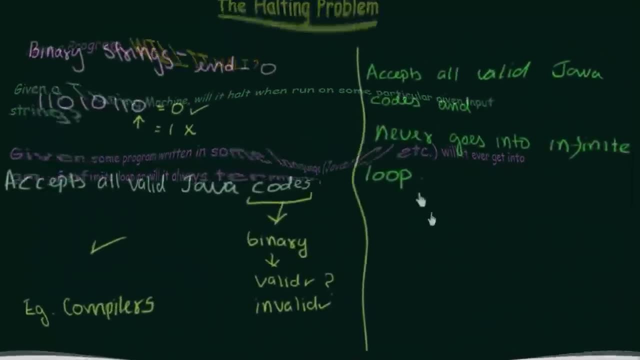 theory of computation and I said that we cannot design a machine that will not allow the code to go into an infinite loop. Now let's just take a glimpse of that lecture. So this was a lecture and I asked that: can we design a machine? 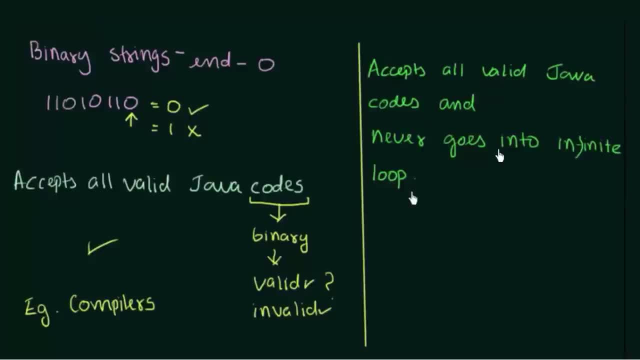 that accepts all valid Java codes and never goes into an infinite loop. So it is of course possible to design a machine that will accept all valid Java codes, but when we include another condition, and that is the program should never go into an infinite loop, I said that it is not possible. 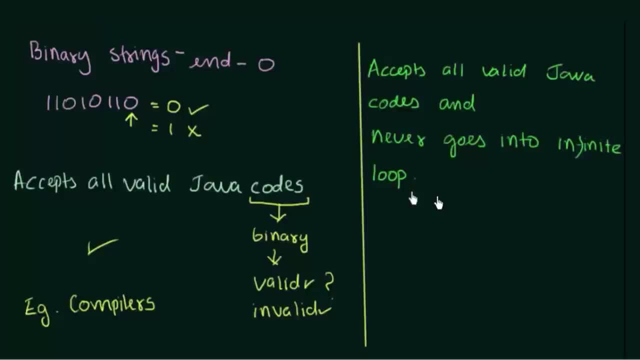 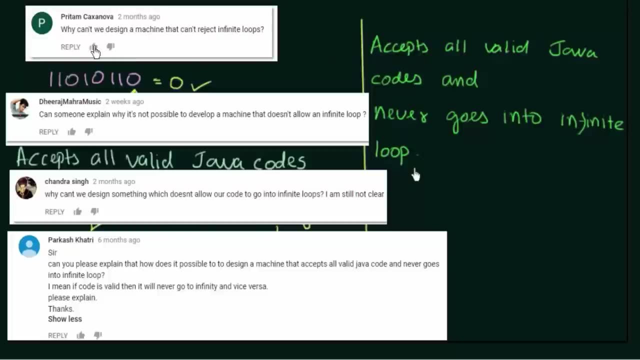 to design this kind of a machine and there were many of us asking why this is not possible. So I got many comments in the comment section of that lecture where many of you asked questions like why can't we design a machine that can't reject infinite loops, or 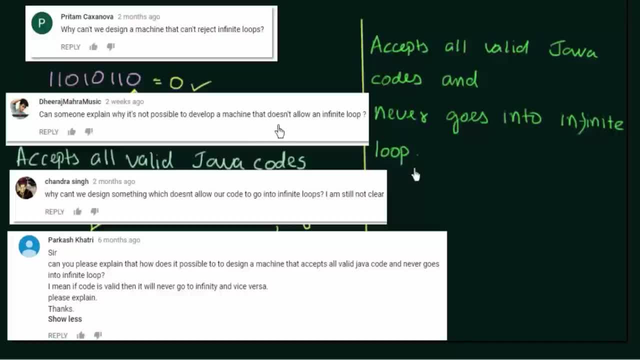 can you explain why it is not possible to develop a machine that does not allow infinite loop, and why can't we design something which doesn't allow our code to go into an infinite loop? and all these infinite loop questions were there, but I did not give you. 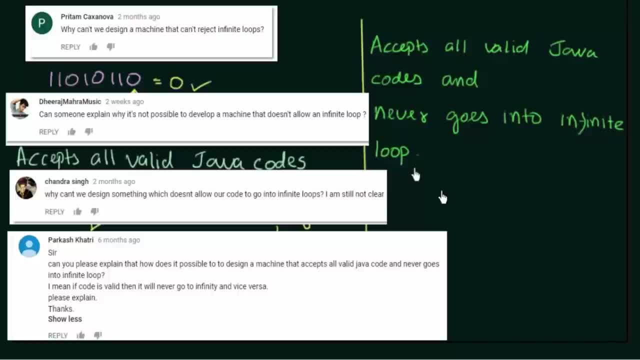 the answer to that question in that lecture, and that is because, in order to understand this, we need to know about undecidability, and we also need to know about how Turing machines work. So now, as we have already covered the topic of Turing machines, 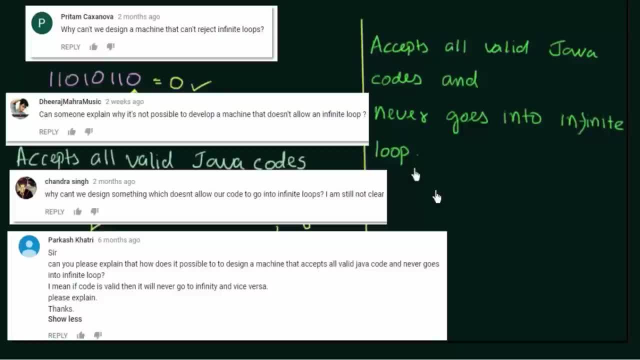 and now, as we know about Turing machines, and also now as we are studying about undecidability and we have the idea of undecidability, we are in a position to answer this question. We will now see. why can't we design a machine that accepts all? 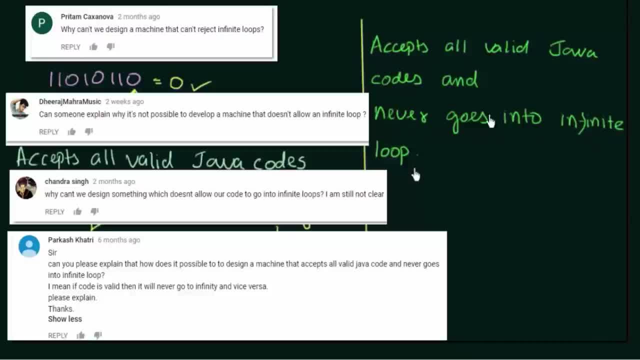 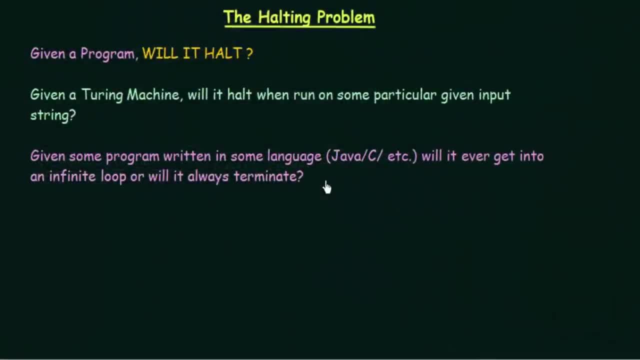 valid Java code and never goes into an infinite loop. This second portion is the important one. So let us go back to our halting problem. So, as I already told you, this is an undecidable problem. The halting problem is an undecidable problem. 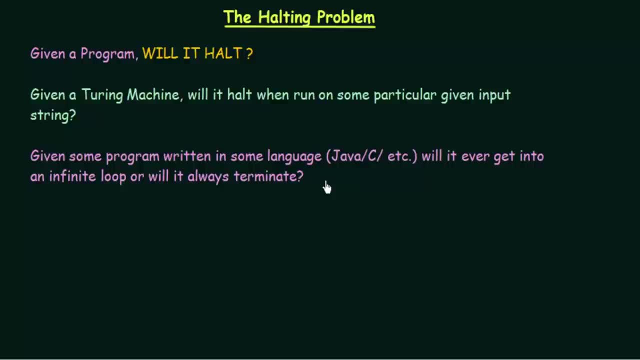 because we cannot have an algorithm which will tell us whether a given program will always halt or not in a generalized way. So the question that we had in the first lecture about designing a machine which will accept all valid Java codes and never go into an infinite, 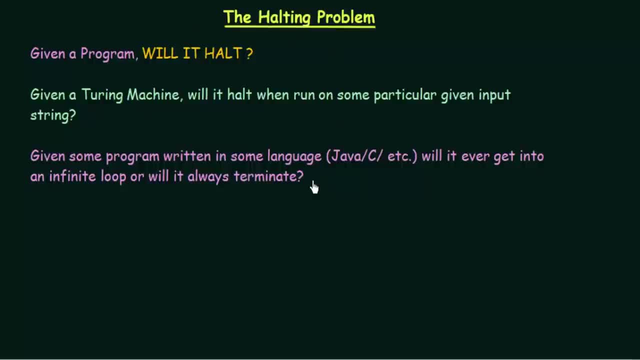 loop is actually the halting problem. Now let us see some answers to these questions. So the answer is: in general, we can't always know. The best we can do is run the program and see whether it halts. For many programs, 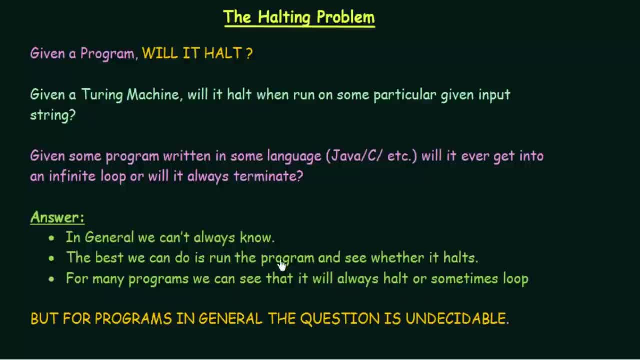 we can see that it will always halt or sometimes loop. So in a generalized way, we cannot know. We can look at some particular programs, as it is shown here, and we can look at the program and we can run the program and see that it is not going into an infinite loop. 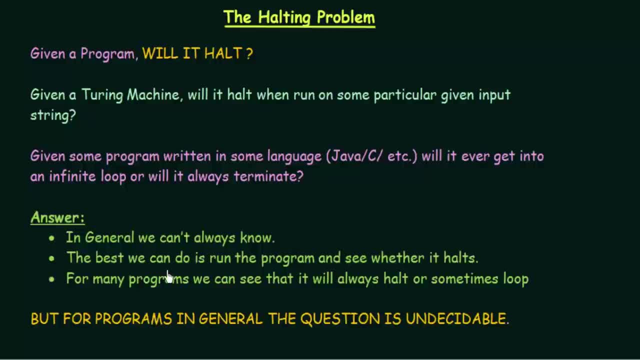 or it is going into an infinite loop. So the only thing or the best thing that we can do is to run the program and see whether it halts or not. But this is not a conclusion. This is just a testing and we cannot. 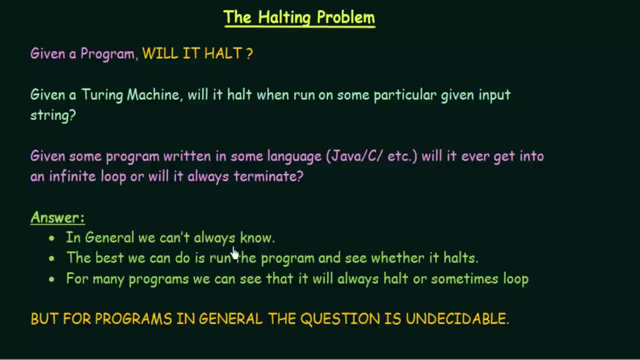 come to a conclusion by this. So in general we cannot know this. For many programs we can see that it will always halt or sometimes loop, But for programs in general the question is undecidable. So we see that this halting 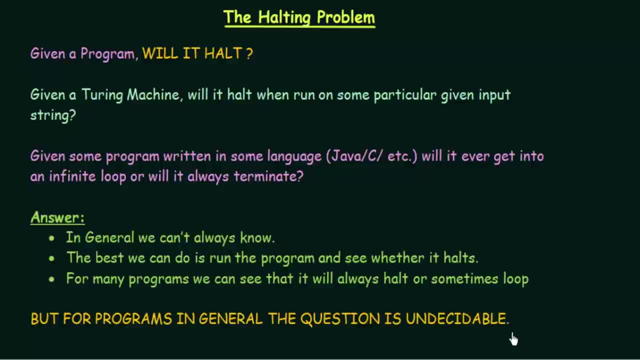 problem is undecidable. Now, if it is undecidable, that means there is no Turing machine that can be designed to solve this problem. We have already seen that in the topic of undecidability when we studied that topic Now from the Church Turing thesis. 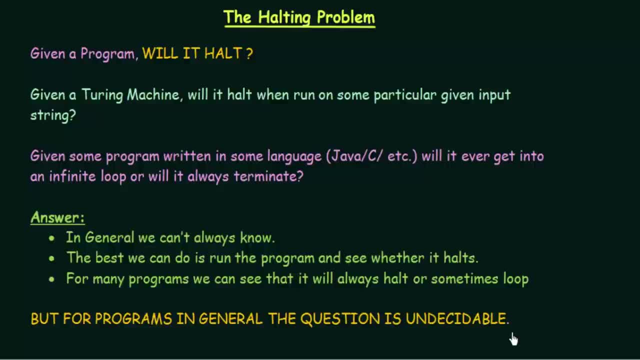 we have already studied that anything that is computable or anything that has an algorithm can be designed using a Turing machine. Now, if you think of that in the reverse way, we can say that if there is a Turing machine for a particular task, then that will have an algorithm.